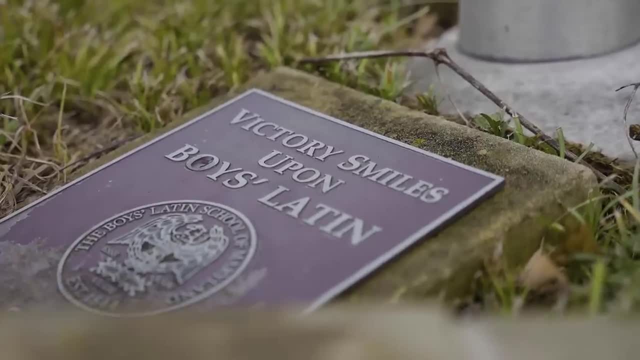 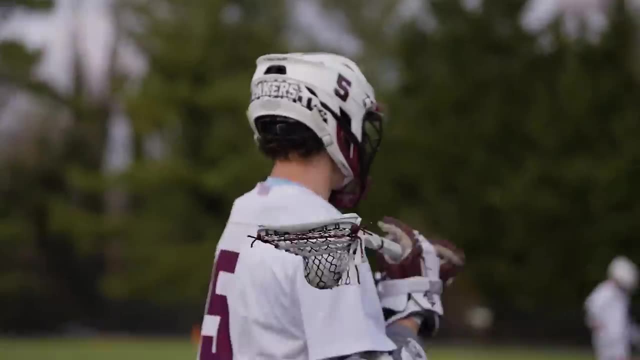 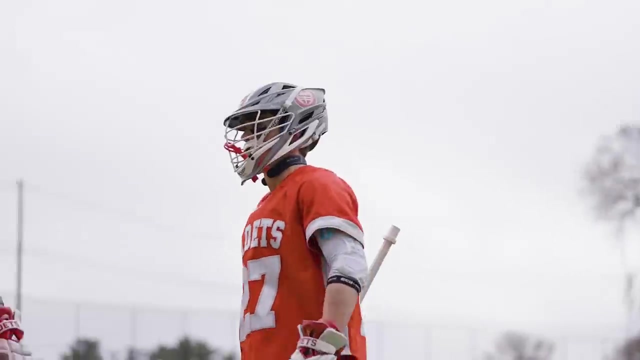 We earned our jerseys, so every play we're 110%. Last week we got humbled, but not this week. And you know what's good about tonight? It's a fresh slate, It's a fresh game. None of that matters. The three things we need: head, heart hustle. Let's go. 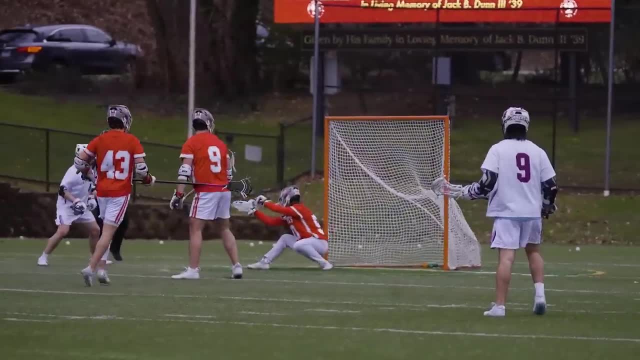 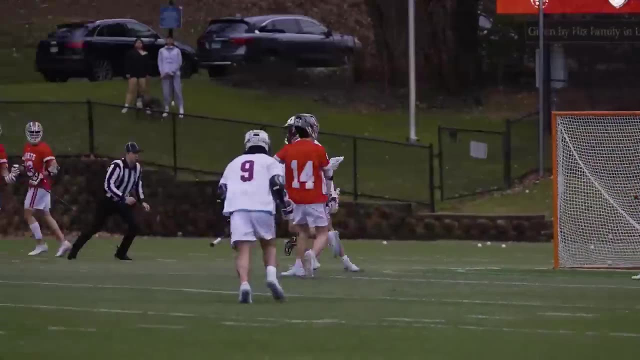 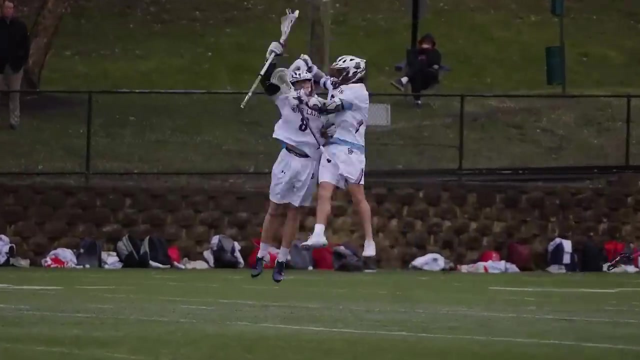 I've got this feeling. on the side of the road, I'd push my car into the bridge. I'm not gonna let it burn. I threw my stock into a bank. I'm not gonna let it burn. I'd push my car into the bridge. I don't care, I don't care. 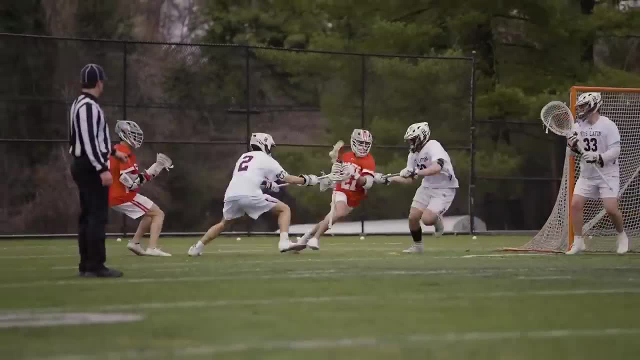 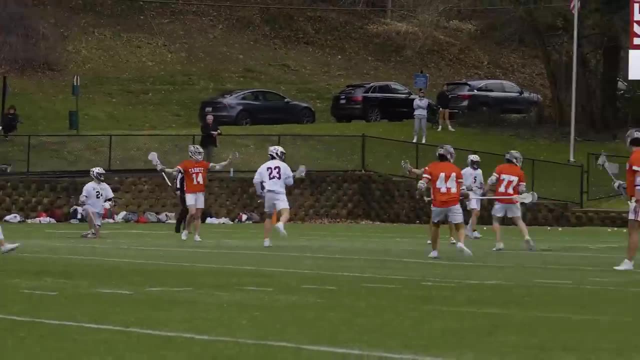 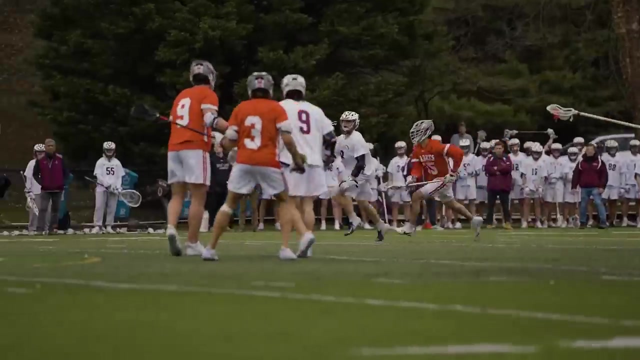 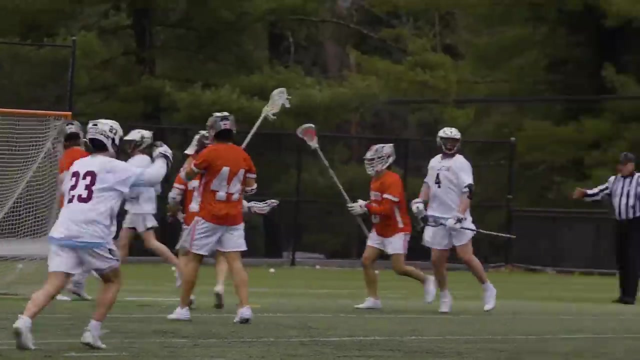 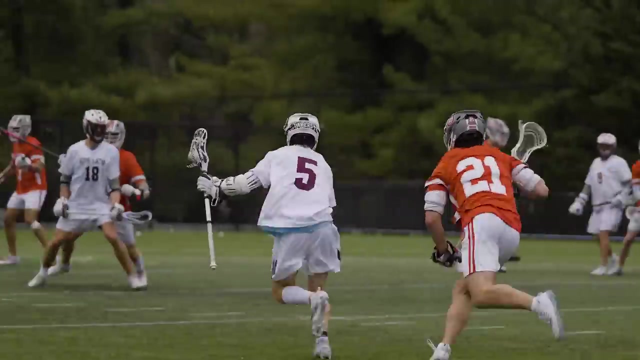 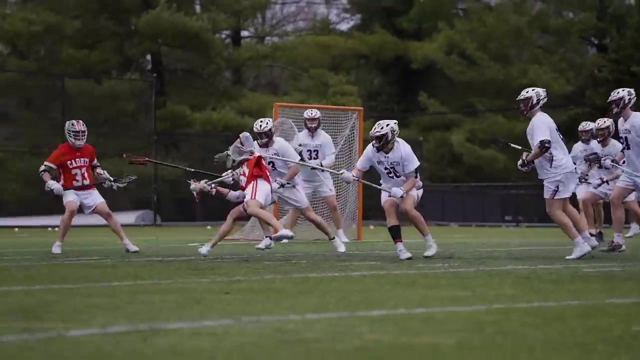 I don't care. You're so close, We gotta kill this switch. You're from the 70s. I love it. I love it. I've got this feeling on the side of the road. I'm not gonna let it burn. I threw my stock into the bridge. I don't care, I don't care. 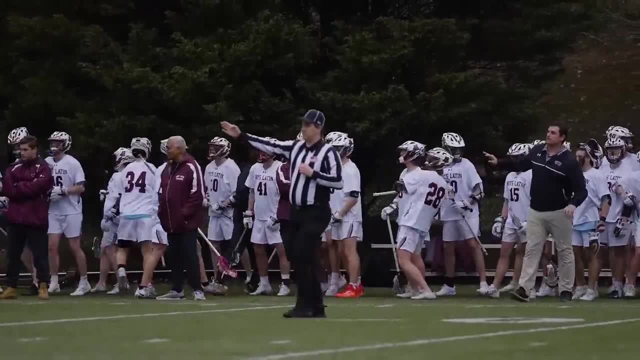 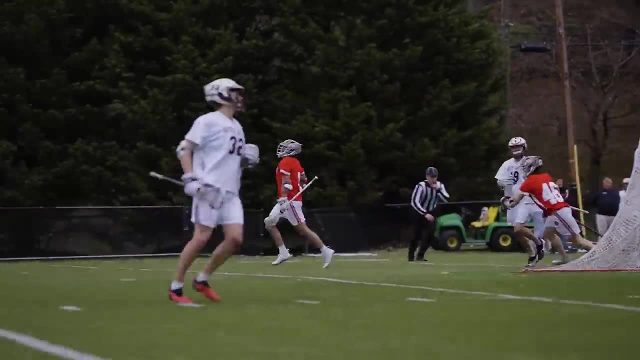 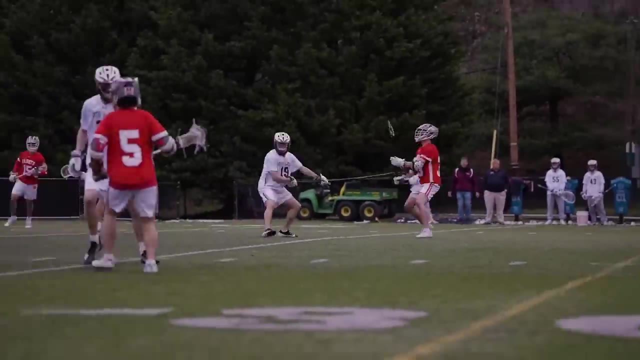 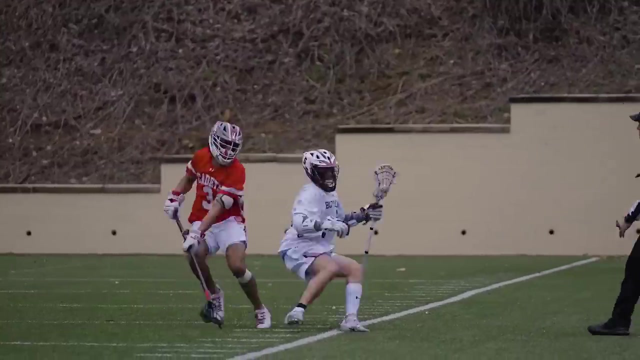 I threw myself into a bag and pushed it down the stairs. I turned my car into the red. I don't care, I don't care, I love it, I love it. I don't care, I love it, I love it. You're on a different road. 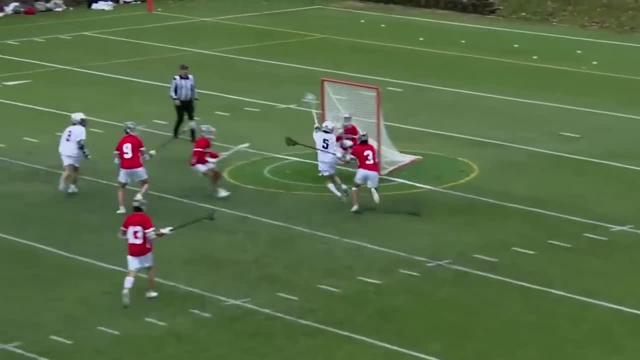 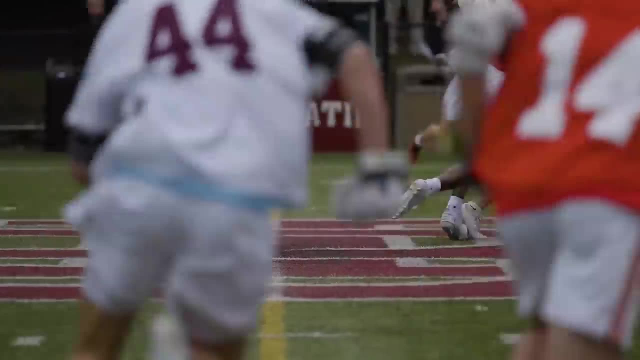 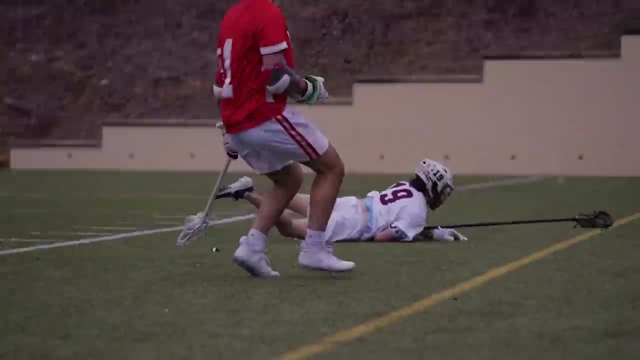 I'm in the Milky Way. You walk me down on earth. I am out of space. You're so hard to face. We gotta kill this switch. You're from the 70s, But I'm a 19th grade. I don't care, I love it. I love it. 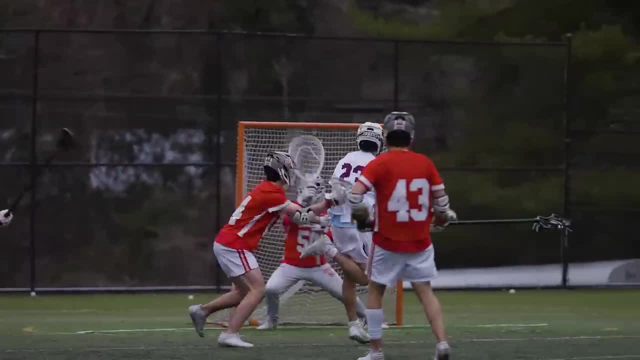 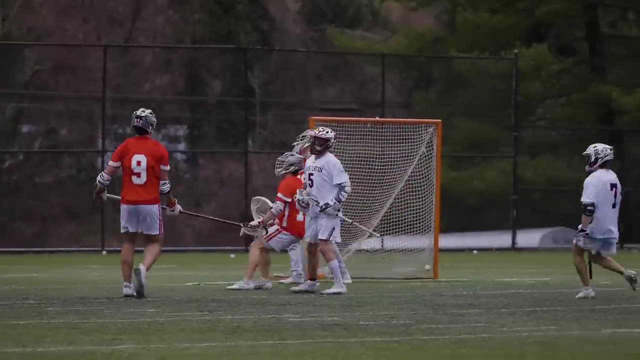 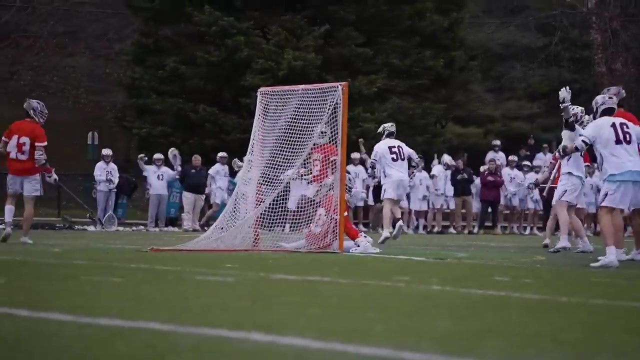